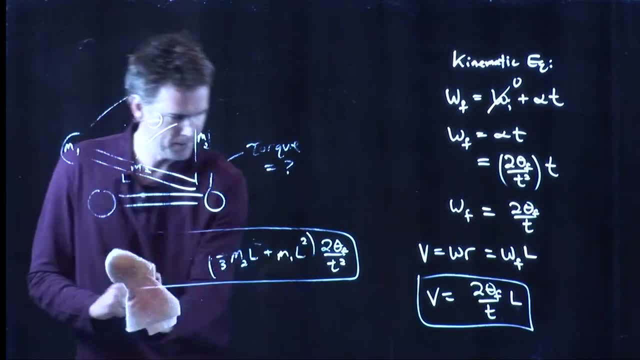 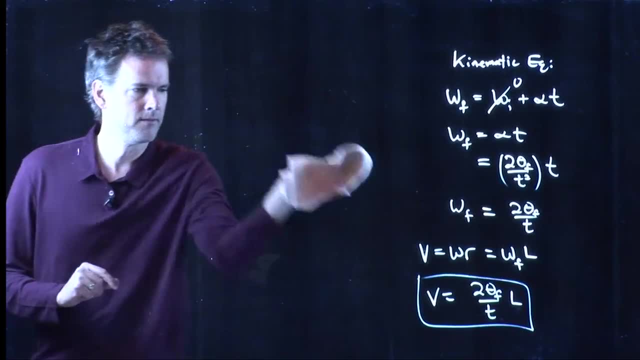 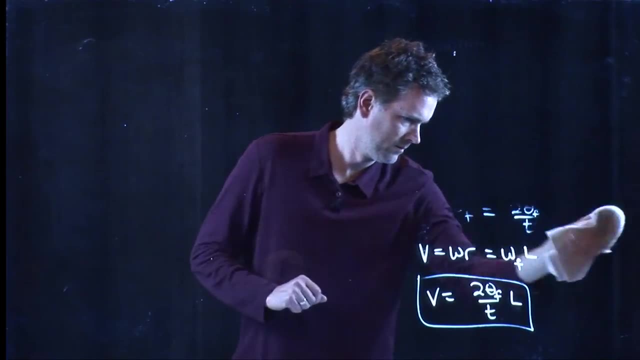 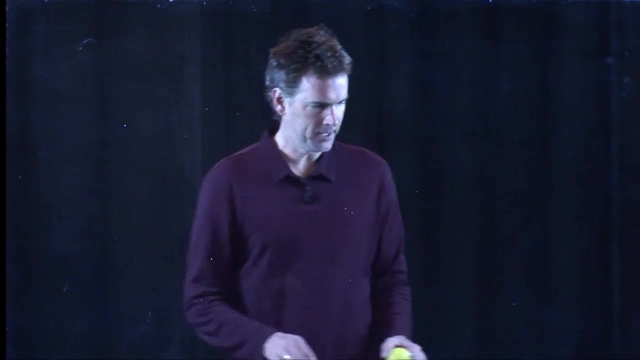 All right, everybody turn to your neighbor, say: hi, My name is, my major is, I'm going to graduate in this year. All right, everybody get to know each other. Yeah, It's good to know each other because some of you might actually give other people jobs one day. 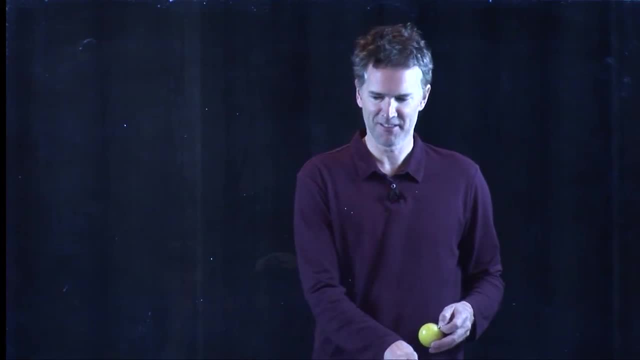 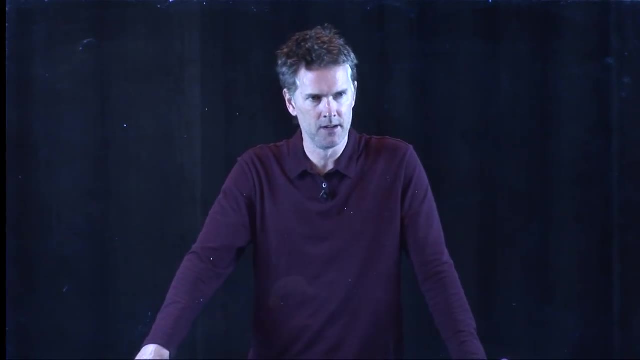 Or you'll need to ask somebody else for a job. It's good to know these people. Okay, hello class. welcome back to another lecture on physics. This is our learning glass approach to lectures on physics. I wanted to talk to you about gravity for a second. 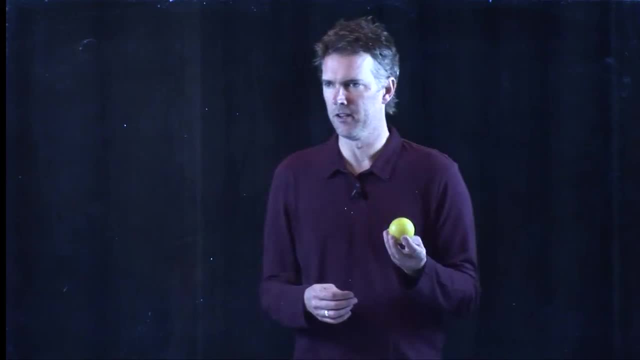 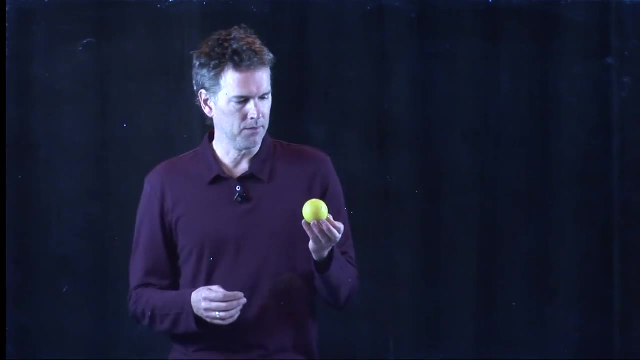 And the Superball is, of course, the best friend of the physicist, And you should just always carry a Superball. You can carry a Superball with you wherever you go. It's just fun to play with. all right, But let's think about the Superball for a second. 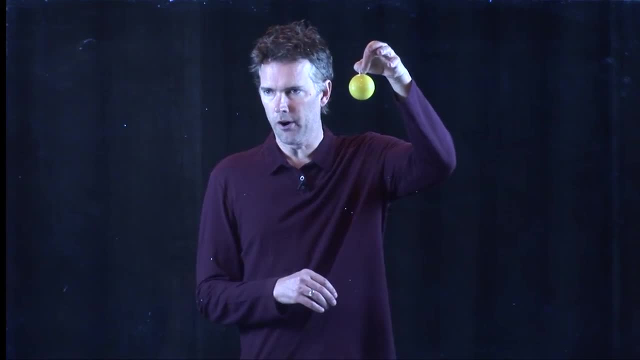 If I hold up this Superball, like so, are there forces that are acting on this Superball right now? What do you guys think? Yes, Yes, okay. What is the net force acting on the Superball? Zero, Why zero? 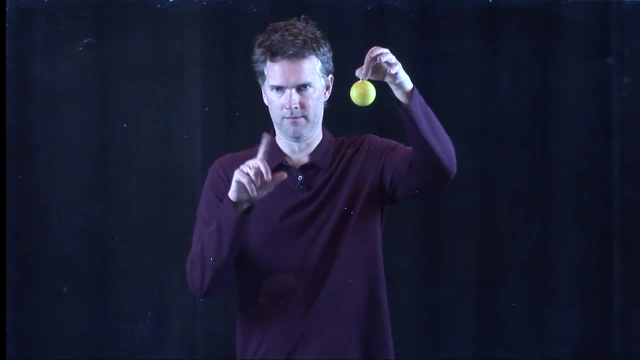 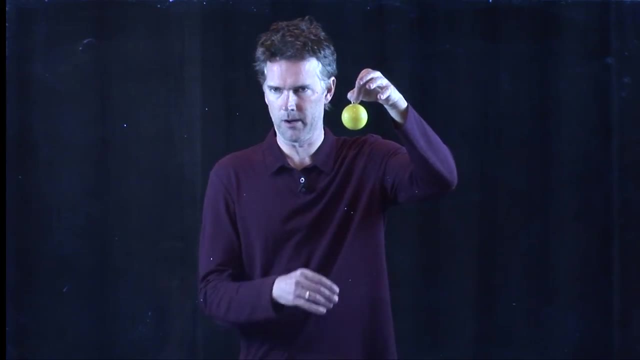 Because it's not moving. Okay, who said zero? What's your name? Adam, Adam. Can you hand the mic back to Adam? Adam and I will have a little chat real quick. Okay, Adam, here's my Superball. 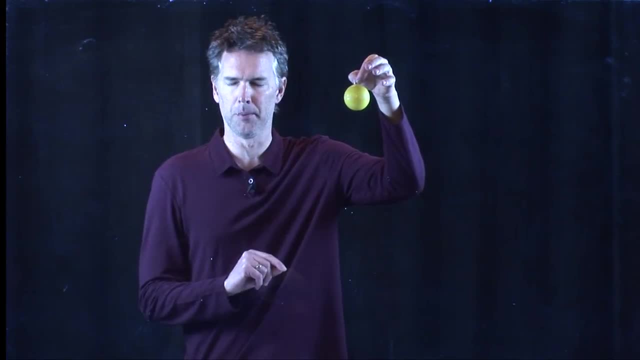 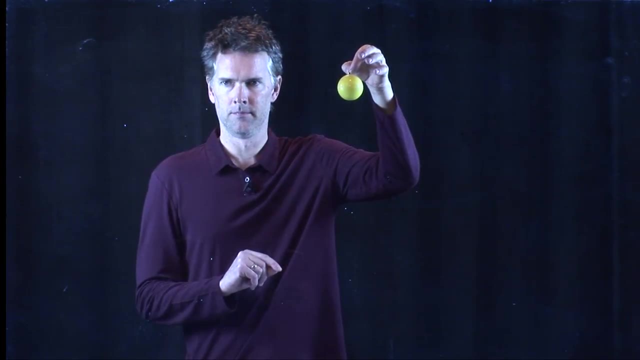 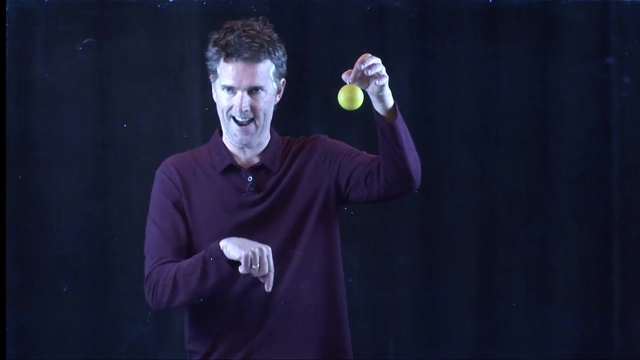 I'm holding it stationary. What's the net force acting on the Superball? Zero Zero. Why? Because there's a normal force applied to it, and gravity as well. Okay, so I'm applying a force, holding it up. Gravity is applying a force down. 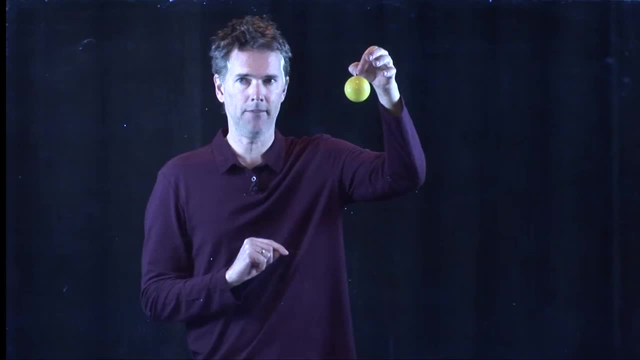 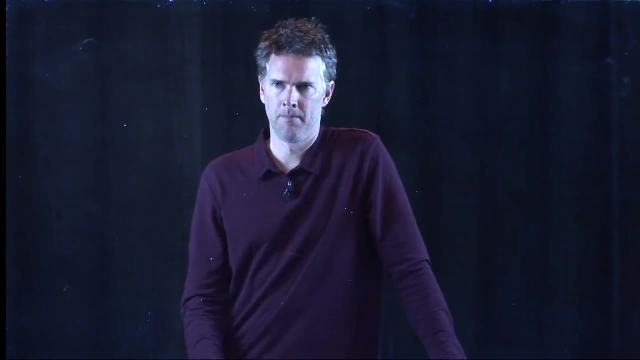 Yeah, Right, So I want to let it go. After I let it go. what was the net force on the Superball before it hit the table, Whatever its potential energy was? Okay, Potential energy is not a force, though, right. 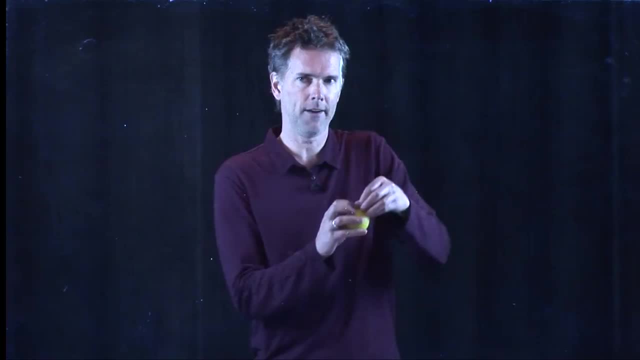 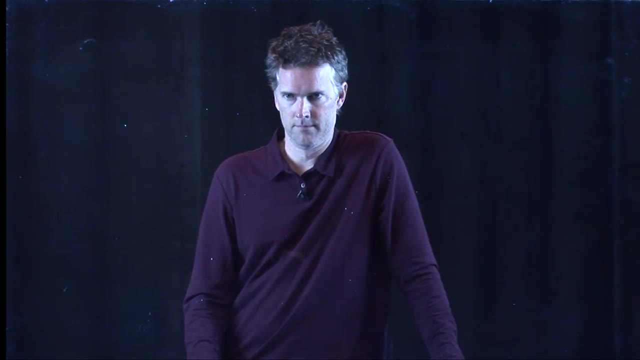 Yeah, It's, of course, related to the force. Yeah, So after I let it go, is the net force on the ball zero? No, No, What is it? It's the force of gravity. It's the force of gravity. 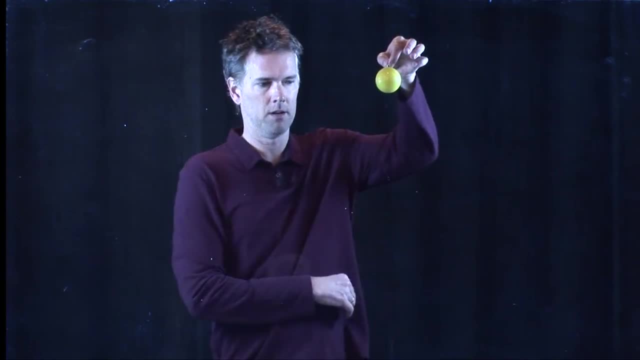 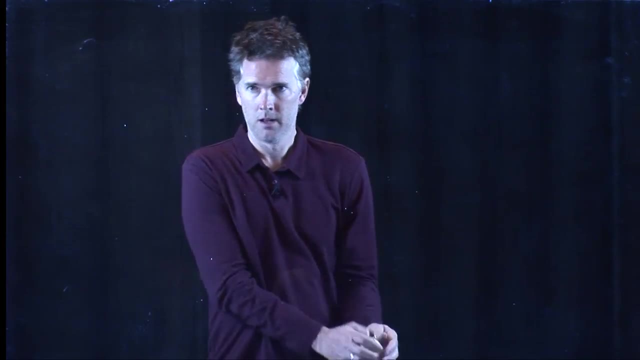 That's right. Okay, So force is zero. I let it go. Force is mg down. Once it hits the table and compresses the bottom of the Superball, what's the net force on it? It's, Is it zero? 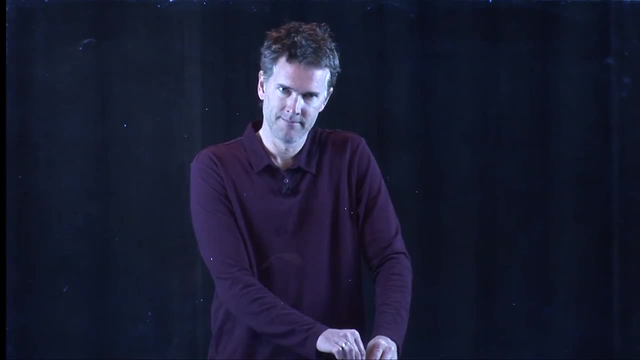 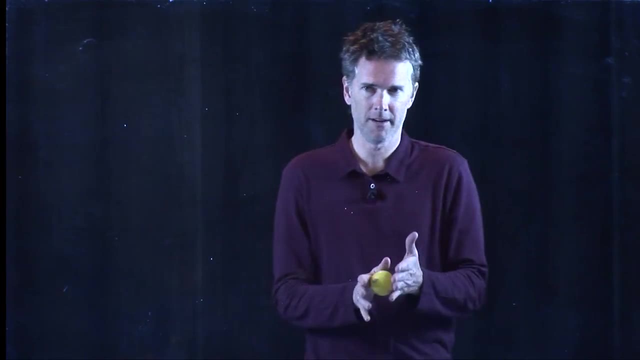 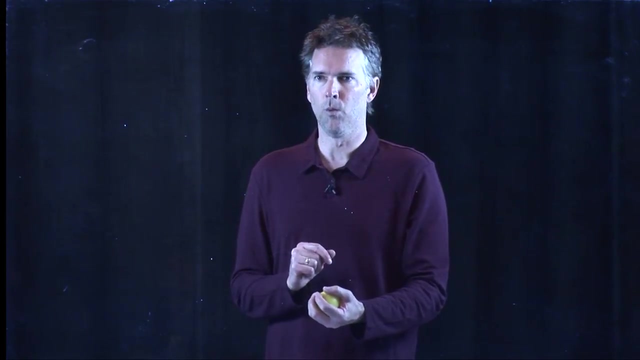 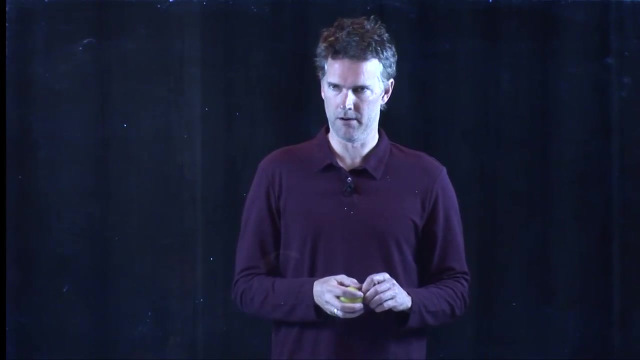 Is it not zero? That's a tough question, right, Let's reverse it for a second. Here's a super ball. It's going to go up. What is the force on the ball at the top of its motion? What is the net force on it? Zero, Okay, why do you say it's zero? 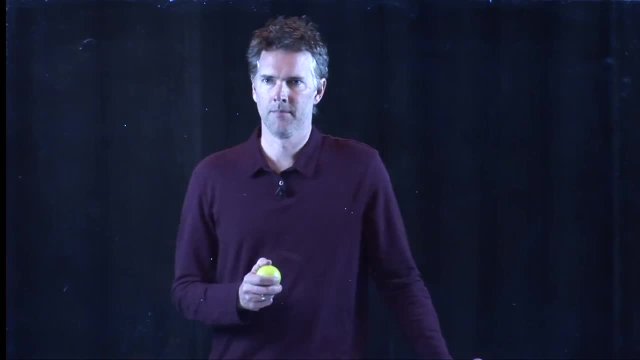 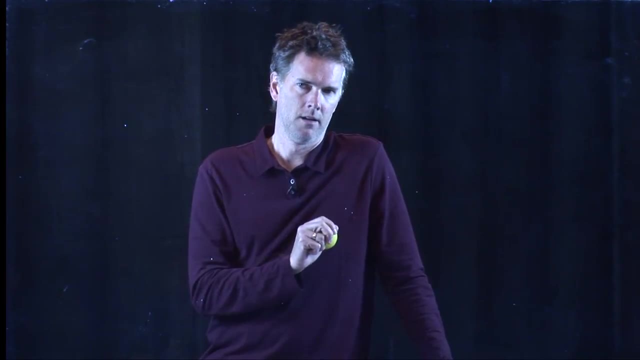 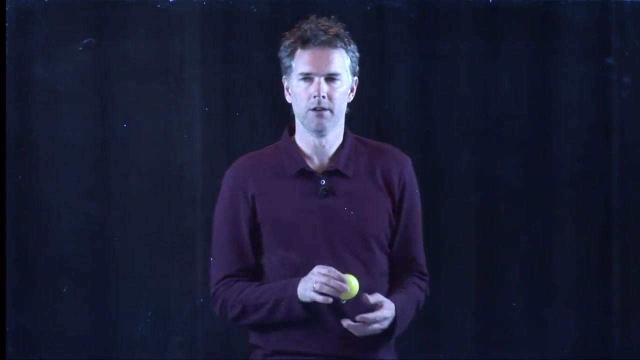 Because for a moment in time it's not moving. It's not moving. Velocity is zero. But what is Newton's second law? Newton's second law doesn't have velocity in it. Newton's second law has what? Mass times acceleration, Mass times acceleration. So does this thing have acceleration at the top of 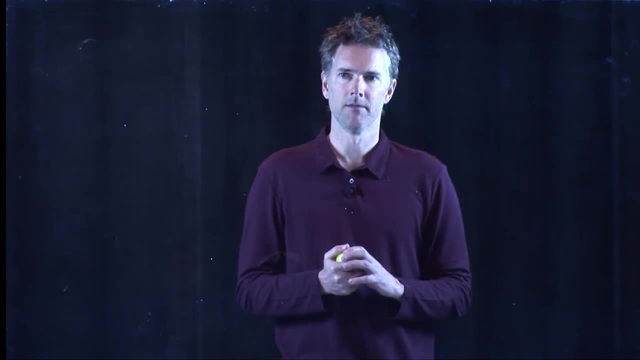 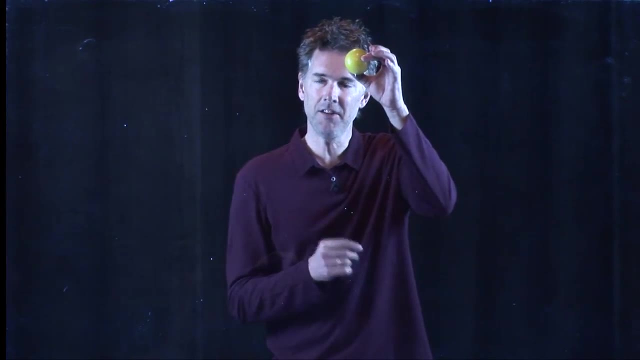 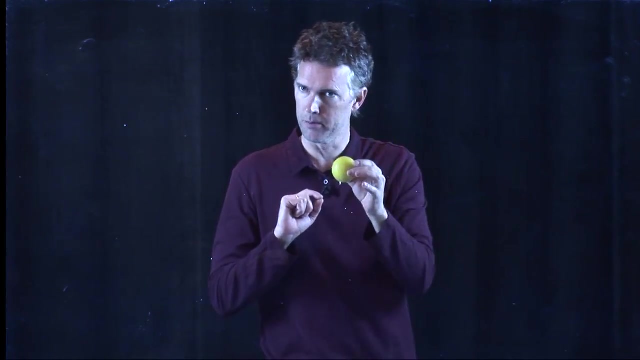 its motion? Yes, Yeah, it certainly does Remember acceleration. is delta V over delta T, In other words, is it about to change its speed? Yeah, Absolutely. It was zero, but we know in the next instant it's going to be falling again. So in 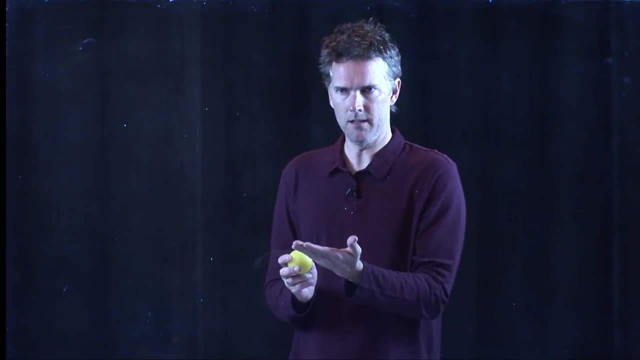 fact, the super ball, as soon as it leaves my hand, it has zero, It has a force on it due to gravity. that is down while it's on the way up, down when it's at the top of the motion, down when it's going back down As soon as it. 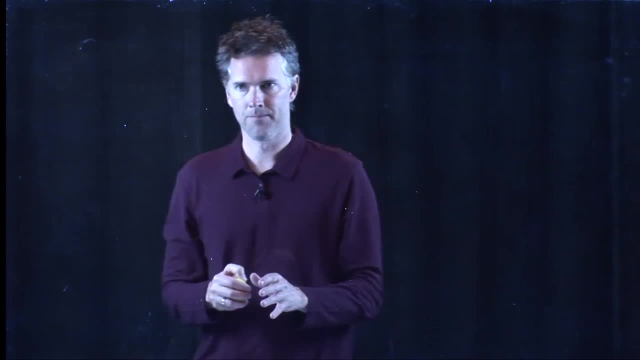 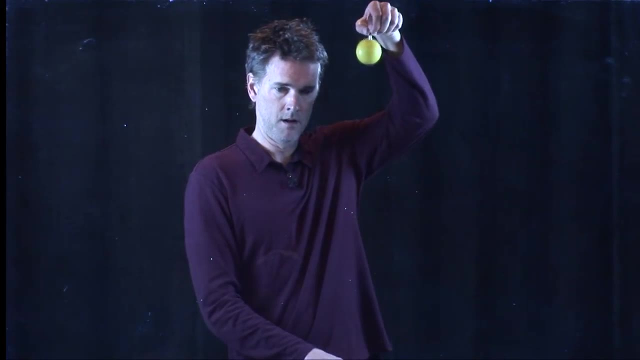 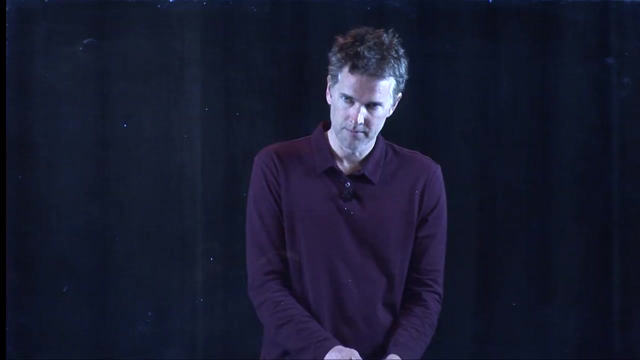 leaves my hand. it's mg the whole time. Okay, so back to the question of when it hits the table here. When it comes to rest and it's in contact with the table, is the force on it zero? or is it not zero, Adam? what do you think? Well, at one point the net force on it is zero, but then the ball compresses a little and I'd say the force is greater than zero. Yeah, exactly right, The ball compresses. It's like a spring is compressed, and when a spring is compressed there is a net force on it. And there is certainly a net force on it when it's compressed, because we know in the next instant it's going to bounce and start to come back. Yeah, 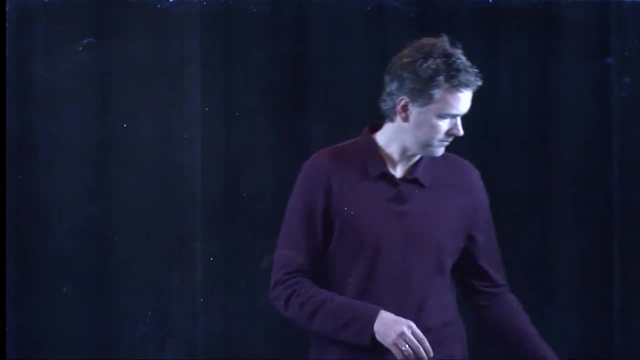 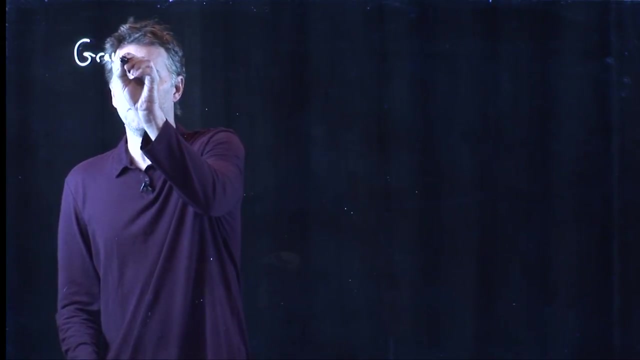 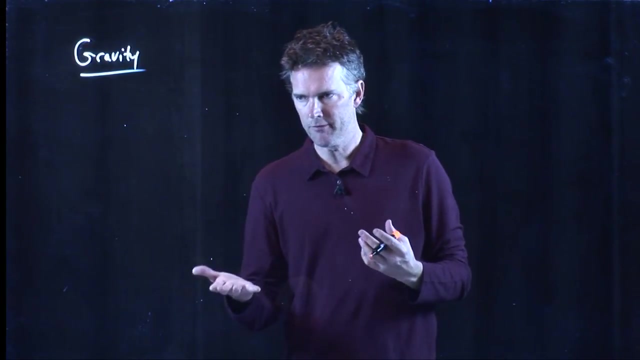 back up. So there is some delta V. All right, fun with Super Bowls. This is all tying into this idea that gravity exhibits a force. Okay, the gravity from the earth pulling down on that Super Bowl made the Super Bowl fall towards. 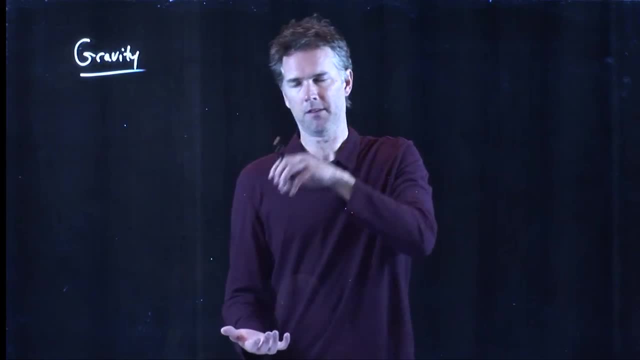 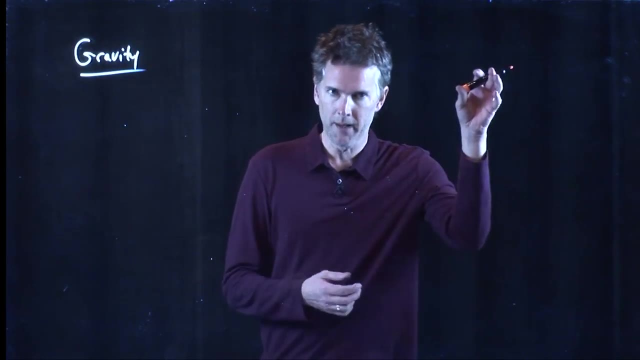 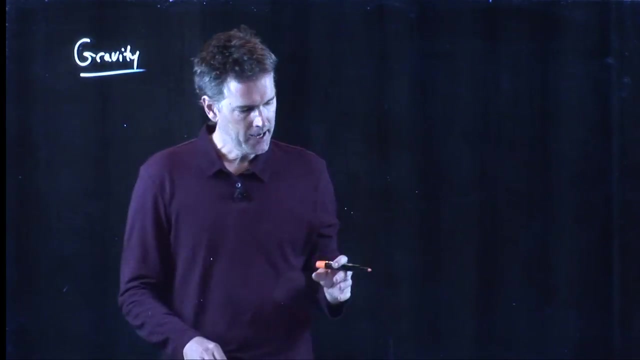 the earth, But it doesn't just apply to the Super Bowl on the earth. It of course applies to you on the earth, Yeah, And it also applies to the moon in its orbit in its orbit and the earth in its orbit around the sun. It applies universally, And this was the huge step. 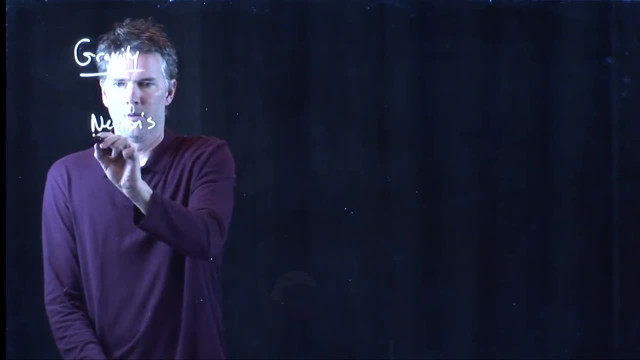 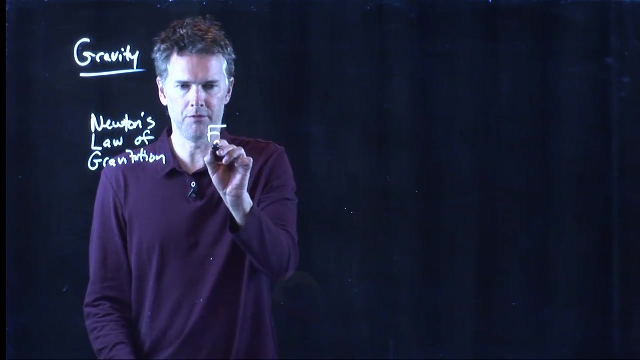 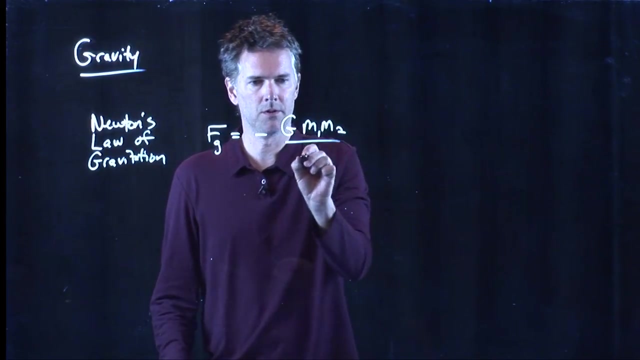 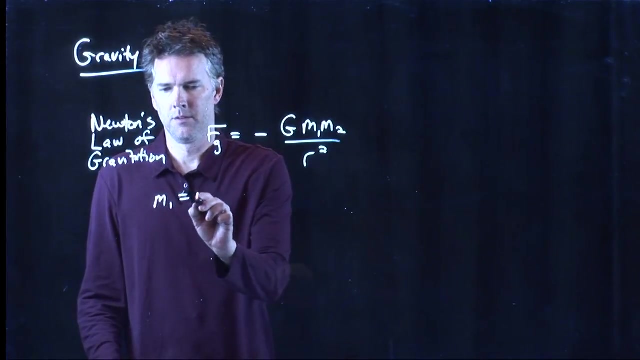 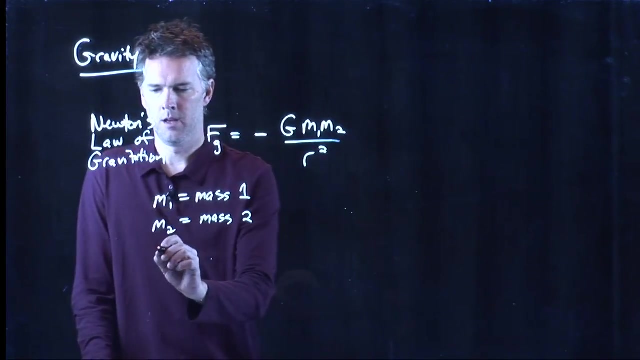 by Newton, which was Newton's Universal Law of Gravitation. Okay, What he said was the following: The force of gravity is negative g m1. m2 divided by r squared m1 is, of course, the mass of one object, m2 is the mass of the other object. So if mass 1 was the earth, then mass 2 would be our Super Bowl G. well, let's do r first. 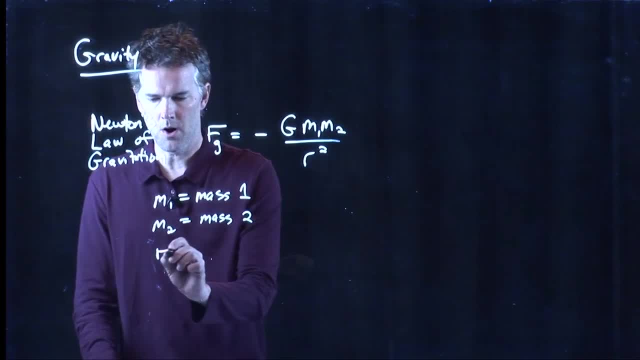 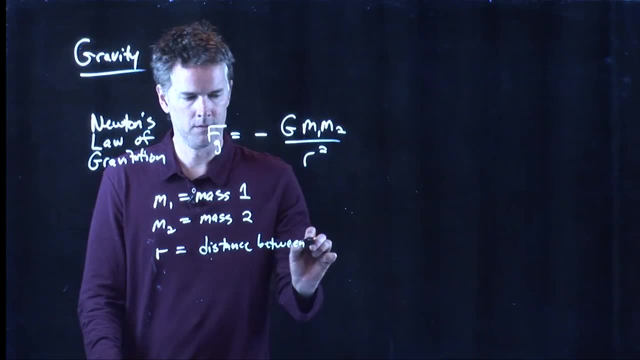 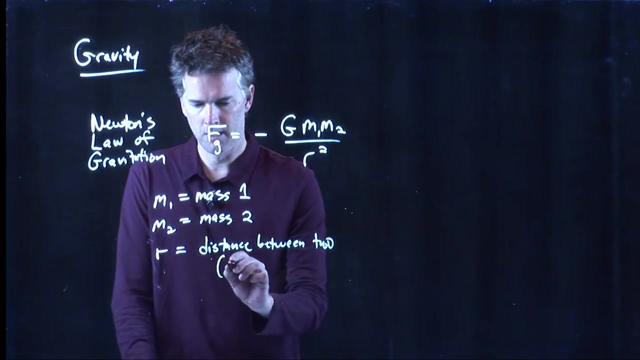 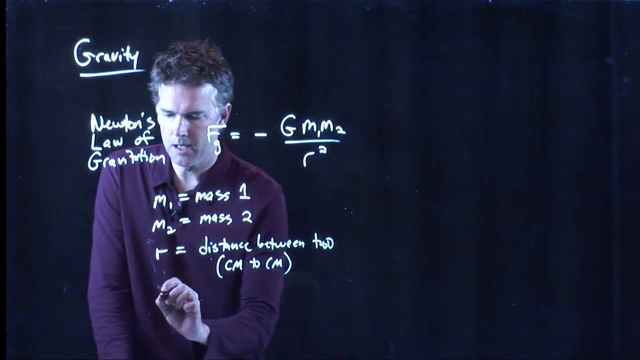 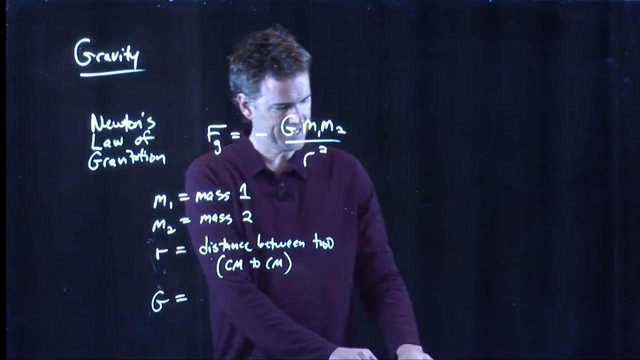 And then we will worry about g. r is the distance between the two, Alright, And if you have spherical objects, then it's center of mass to center of mass, distance. And then, finally, g is the universal gravitational constant, constant, and it has a particular number. We'll give you a few digits here. 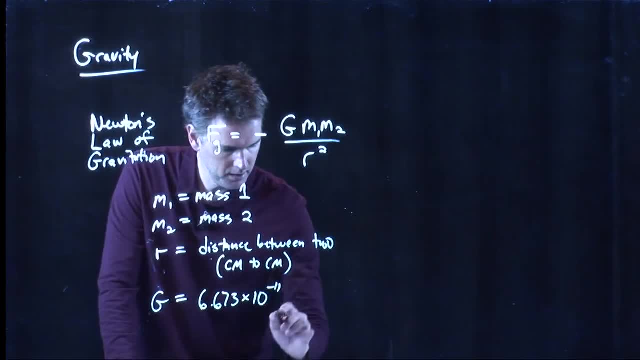 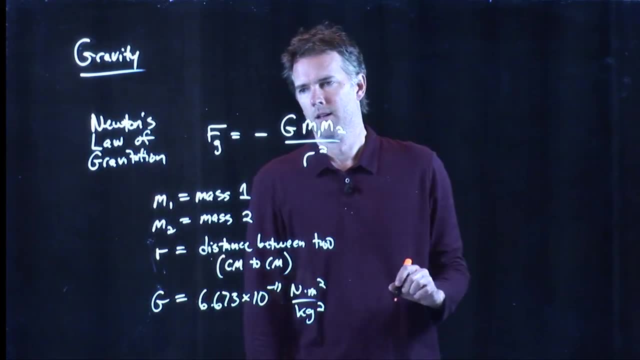 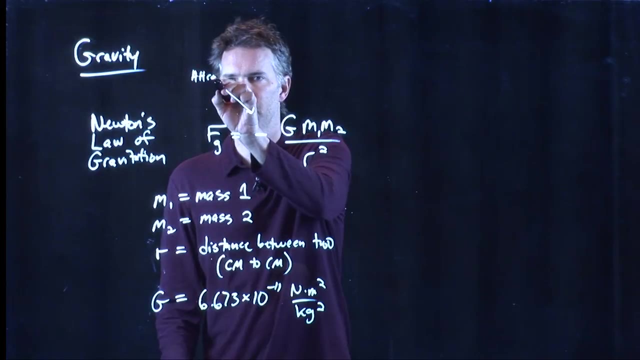 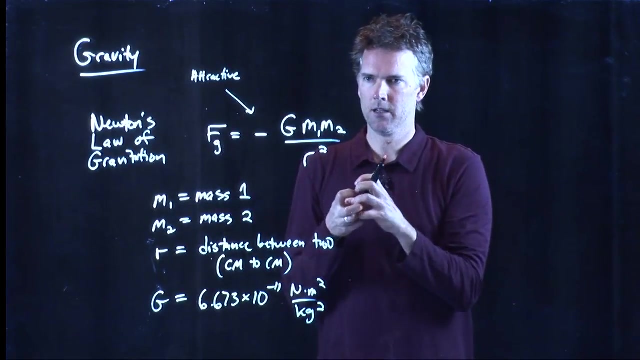 6.673 times 10 to the minus 11 Newton meters squared per kilogram squared. What about this negative sign? That negative sign just means it's attractive. Okay, masses are attracted together, which is a good thing, because if masses, 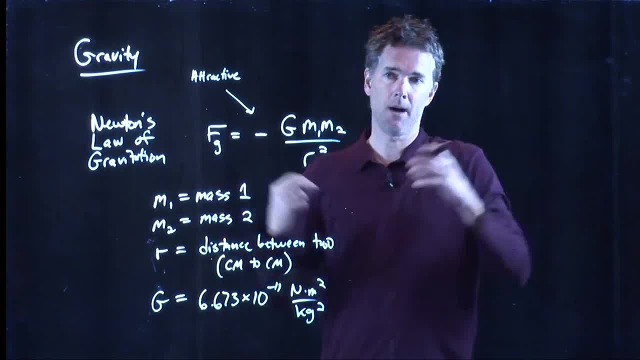 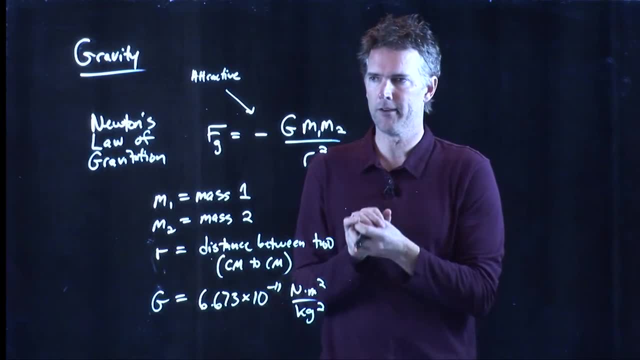 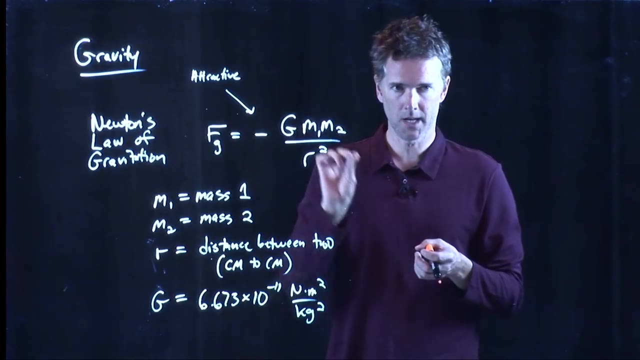 weren't attracted together. guess what? As soon as the Big Bang happened and we had expansion of the universe, stuff would never come back together. Planets would never form, Stars would never form. The only reason that planets and stars form is because gravity is pulling them together. And if none of those stars 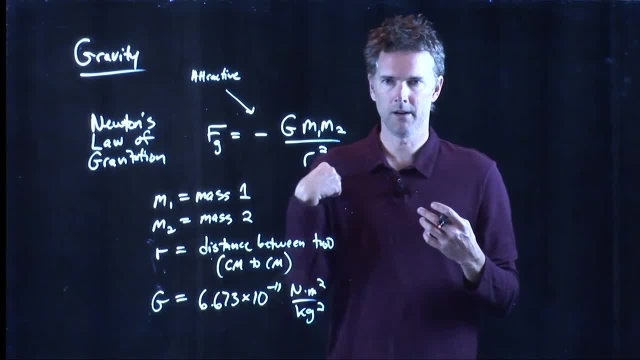 formed and none of those planets formed and none of those planets formed, then you wouldn't be here, I wouldn't be here, none of us would be here, And so we wouldn't have to worry about this universal law of gravitation at all. 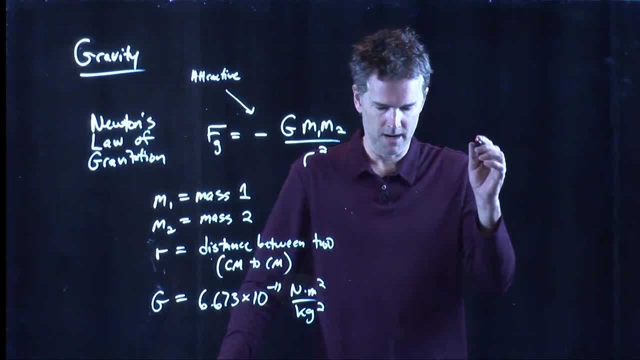 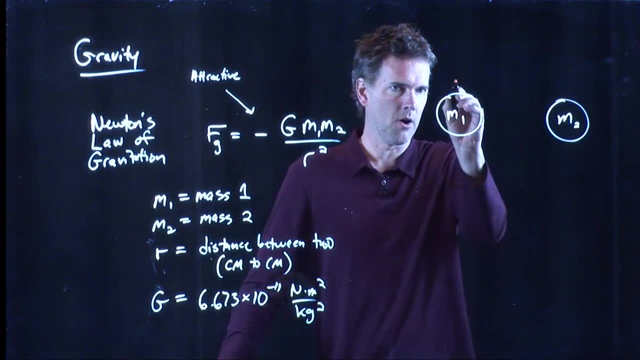 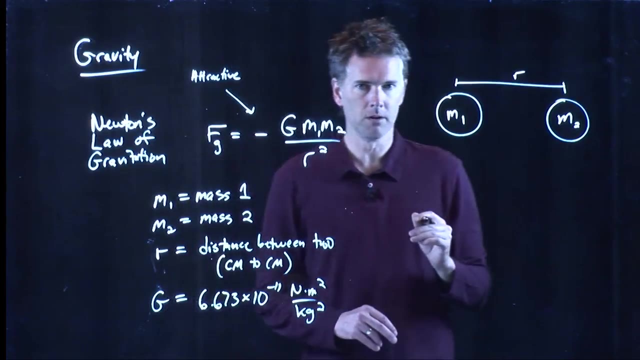 Maybe that would be better, I don't know. It's not too bad. All right, let's think about the two masses here, M1 and M2.. R, we said, if they're spherical, it's center of mass to center of mass, which for a sphere, it's right in the middle of the. 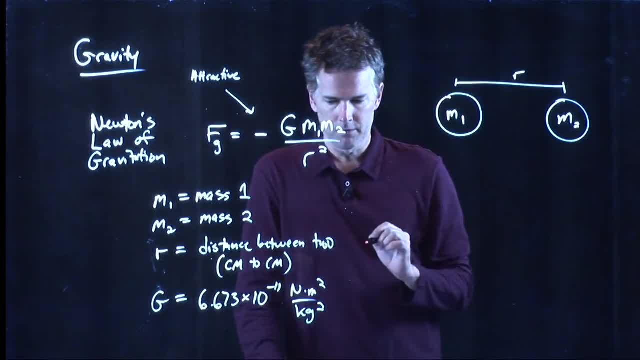 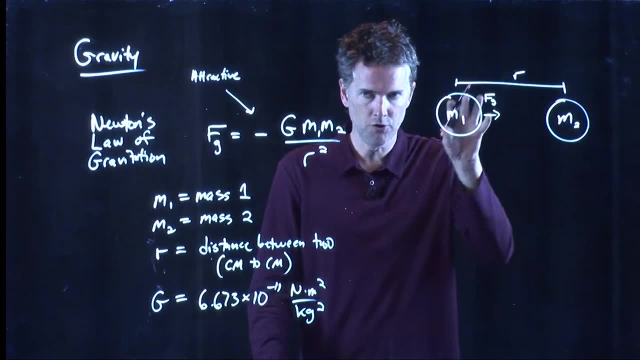 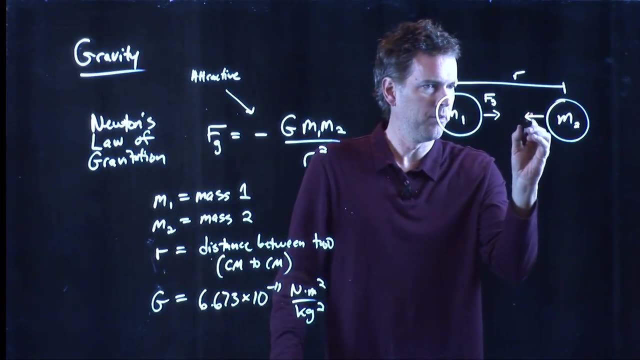 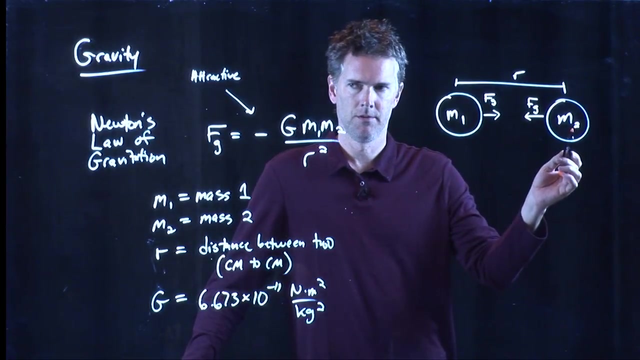 object G is the universal law of gravity, Universal gravitational constant. This says there is a force on M1 due to M2 trying to pull it towards it, But there is also a force of exactly equal magnitude opposite direction on M2.. And we know exactly what that force is: The 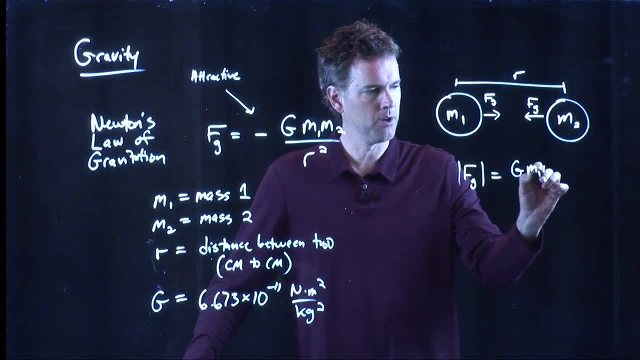 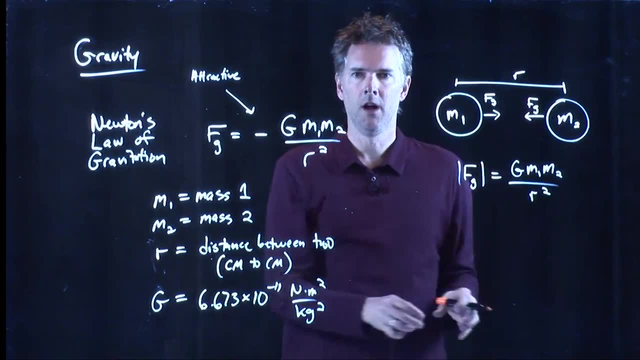 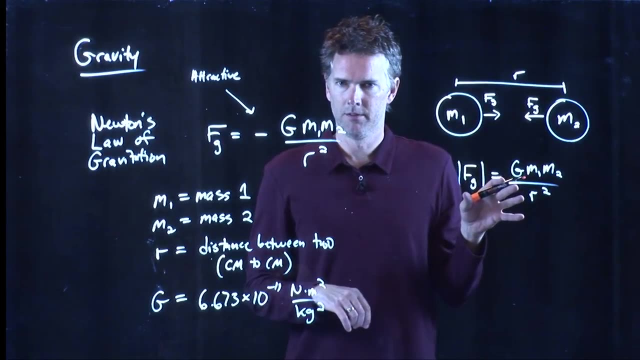 magnitude of that force is g, M1, M2, M2.. Over R, squared, Any two objects in the universe are attracted together by gravity, for any object in the universe, Okay, which is kind of weird to think about, right, Because you're all familiar with being stuck on the earth, right? But 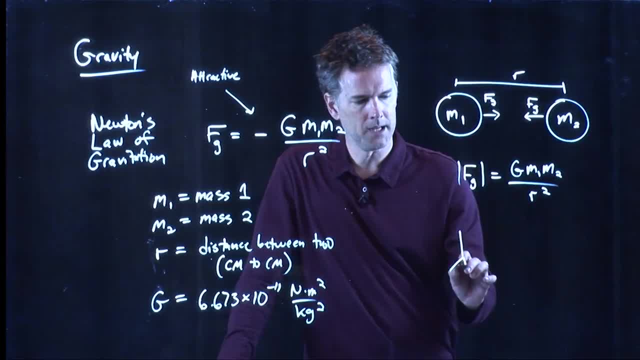 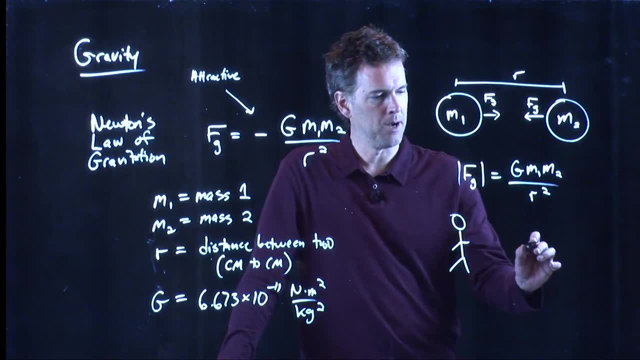 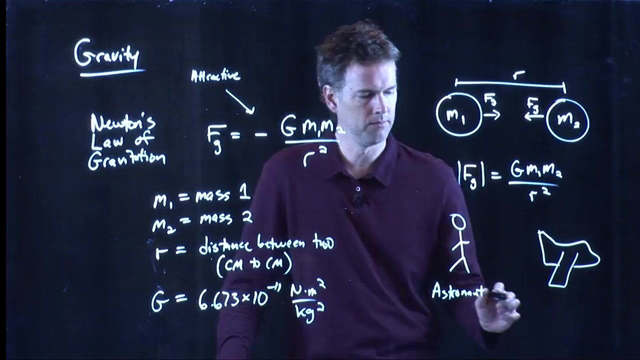 you're not as familiar with being attracted to other objects. So, for instance, if I'm in outer space and my space shuttle is floating over there somewhere and I can't get to it, how do I get to that space shuttle? Well, we talked about this before, with the idea 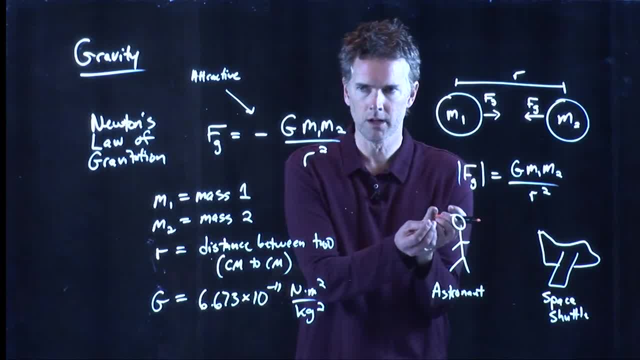 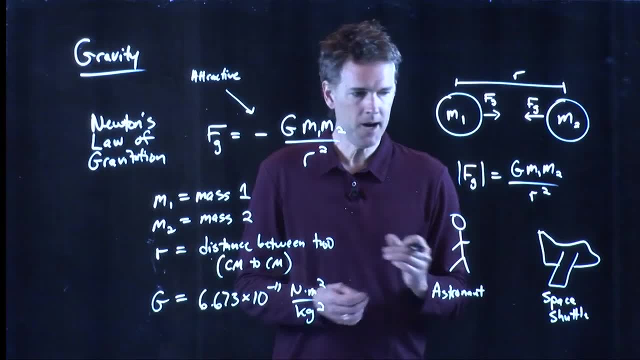 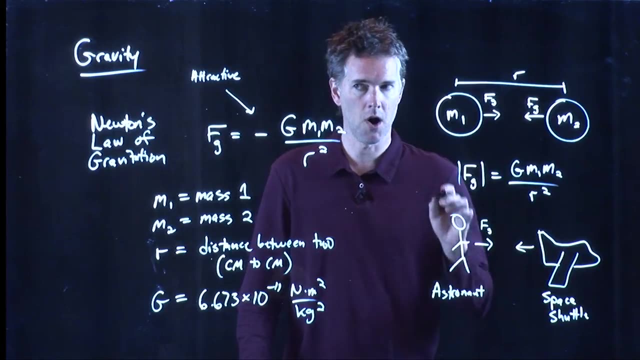 of conservation of momentum. If I had a wrench in my hand, I could throw a wrench the other way and I would be propelled towards the space shuttle. But I could also just wait. There is a force due to gravity on me pulling me.